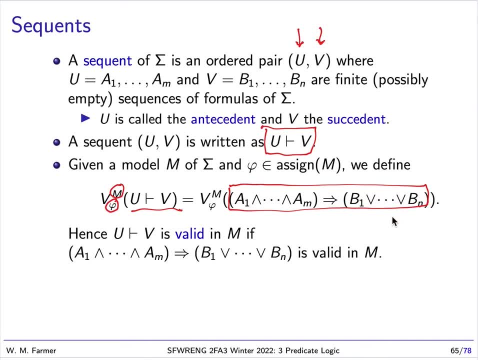 And the formula says that the conjunction implies the disjunction, And for that reason we will say that a sequence is valid precisely if this formula is valid, Or, in other words, it's valid in a model, if this formula is valid in a model. 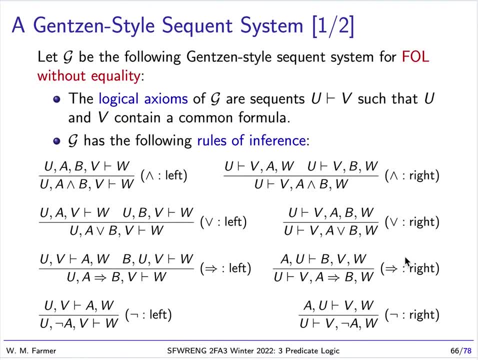 So last time we presented a Jensen-style sequence system for FOL, but I failed to emphasize the fact that it was for FOL. without equality We don't have any machinery for reasoning about equality. And remember, equality is basically a logical constant in our logic in FOL. 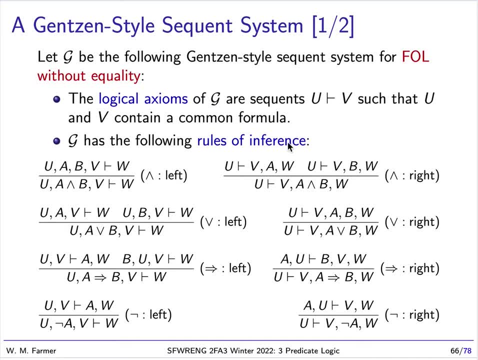 So, anyway, last time we presented this Jensen-style proof system, it had one logical axiom and a whole bunch of rules of inference, And we had rules of inference, pairs of rules of inference for each A Boolean operator and each quantifier, And then we talked about what proofs are. 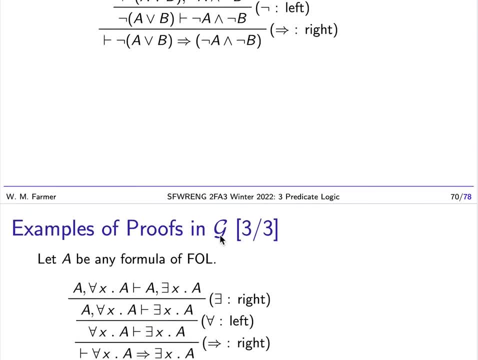 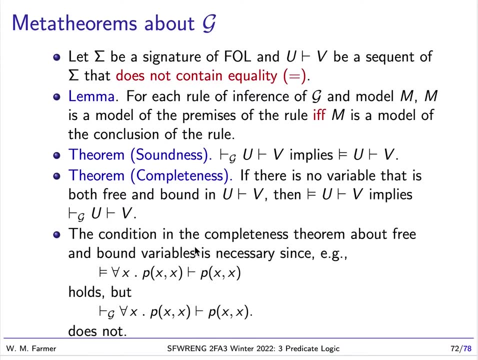 And we gave examples of proofs, several examples. So now we're ready to talk about the metatherems of G, this Jensen-style proof system. So remember, G proves theorems and theorems about G. we call these metatherems. 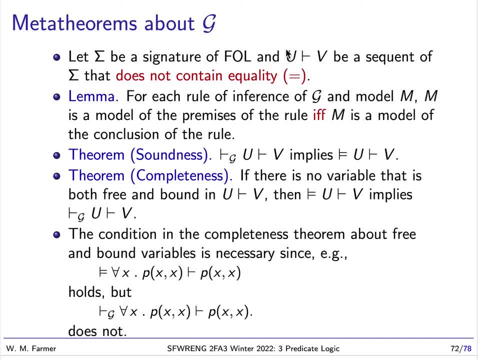 Now let's Our sequent here be any sequent of a signature sigma, as long as that sequent does not include equality. Now, one thing that's true, that's actually quite useful, is that for every rule of inference of G in every model M. 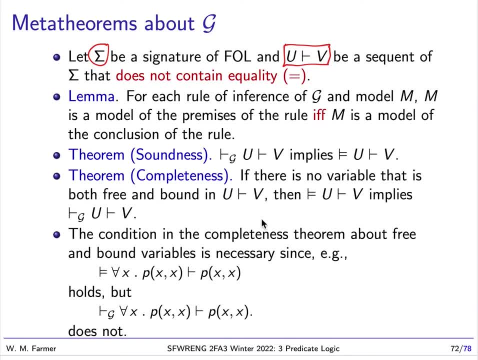 M is a model of the premises of the rule, if, and only if. M is a model of the conclusion of the rule. So this is unusual. Usually we don't have if and only if we have implies. So usually if we have a rule of inference like this, from A and B we can infer C. 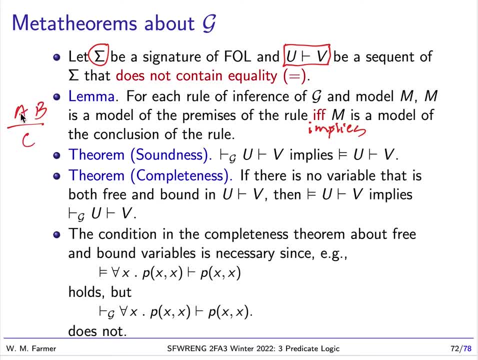 Usually what that means is: if A is valid in a model and B is valid in a model, then C is valid in a model and it doesn't go the other way. So truth flows in only one direction, So usually So truth flows in only one direction. 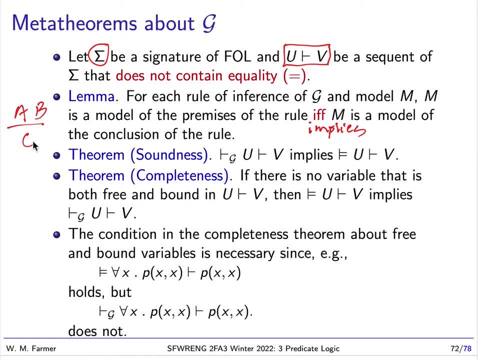 So usually, So usually, if C is valid in a model, that does not mean necessarily that both A and B are valid. But in this case we have if, and only if, We have truth flowing both ways for our rules of inference. 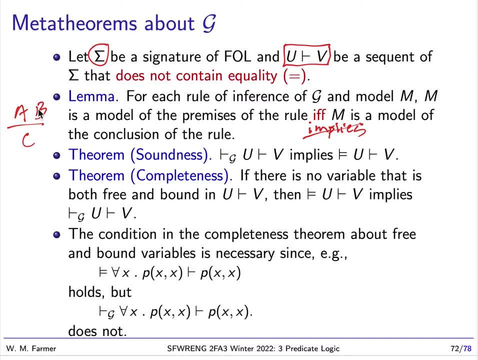 If we have a model of A and B, then that will be a model of C, and if we have a model of C, it will be a model of A and B. Now we also have two very nice theorems: Soundness and completeness. 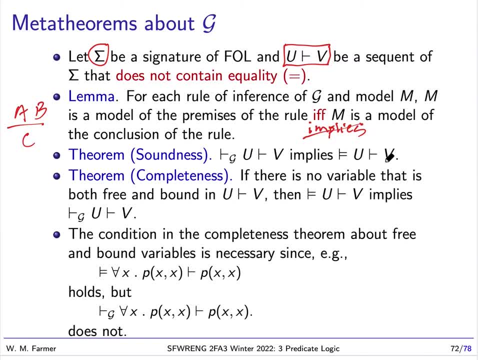 Soundness says: if we can prove this sequent, that implies that that sequent is valid. In other words, it's going to be true, it's going to be valid in every model And we have completeness which says that if the sequent is valid, then there will be a proof of it. 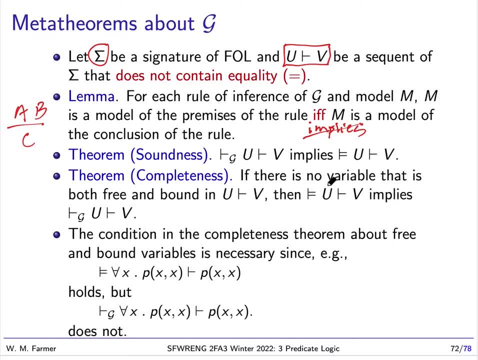 Now this completeness theorem requires that no variable is both bound and fruit, And that's really not much of a restriction, because you can always write down the formulas you want to prove, without using a variable, as being both bound and free. So I want to illustrate why this happens. 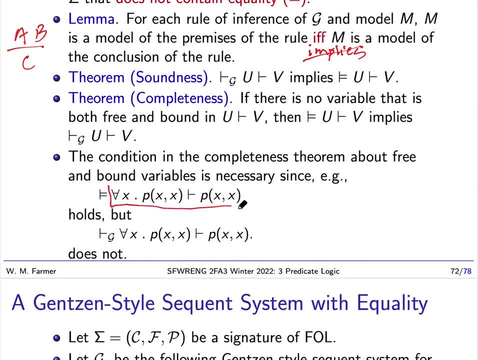 If we look at this formula, this is clearly valid because it says that for all x, P of x, x holds. It says that this holds will imply that P of x- x holds. Now, the reason this is true is because if a universal statement holds, then every instance of it in P of x- x is an instance of for all x, P of x, x. 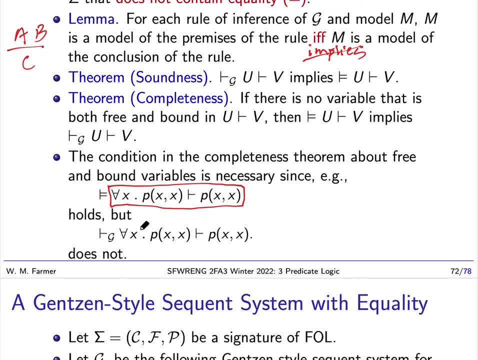 But now if we're trying to prove this. so if I was going to start with this and trying to prove this sequent I'd probably want to use. the only thing I can use really is for all left. 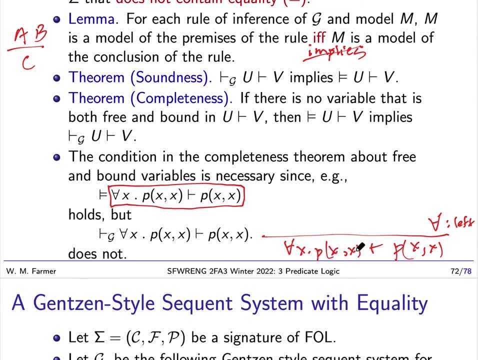 Now for all left says I can replace x with any variable that's not free in here, free anywhere else. Well, the variable I want to replace x with is x. That way I can get get this And that will be a logical axiom and I'll be done. 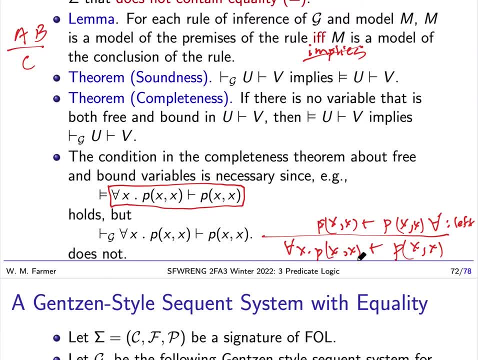 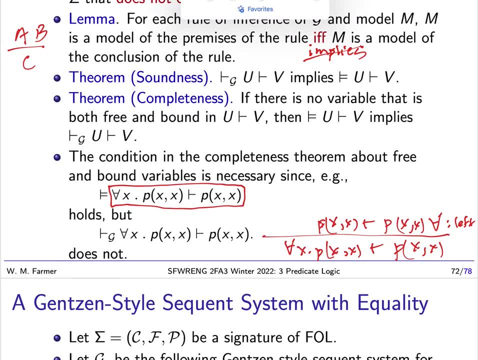 But the problem is I'm not allowed to replace x with x because x is free, So so what we get here? let me use a different color. This does not work, So we can't. there isn't a way of proving this. 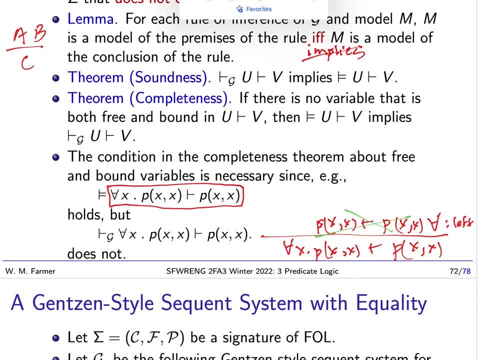 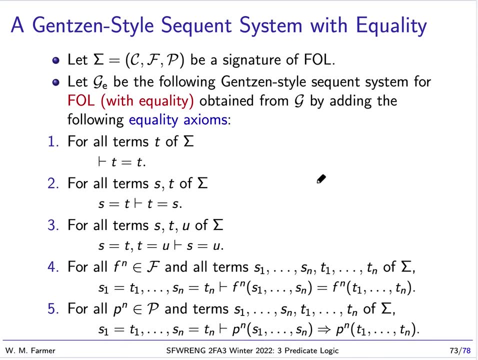 But, like I said, this is not a big deal because we can always start with our variables either being all free or all bound. Okay, so I mentioned that this system, g, doesn't work with equality. We can modify g, so it does work with equality. 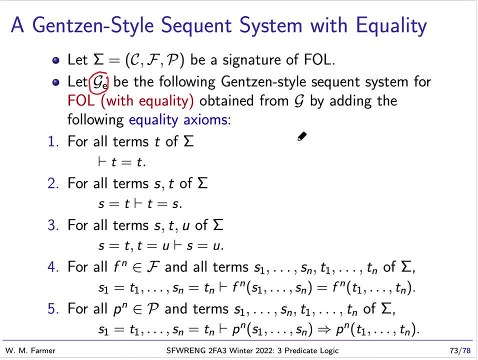 We get g sub e. This works perfectly well with equality, but we have to add some more axioms. We have to add axioms that are similar to the axioms that we had for our Hilbert-style system h. So we have. 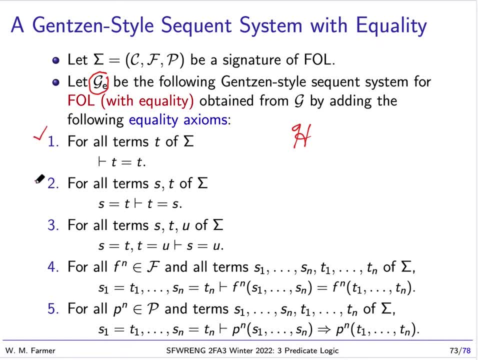 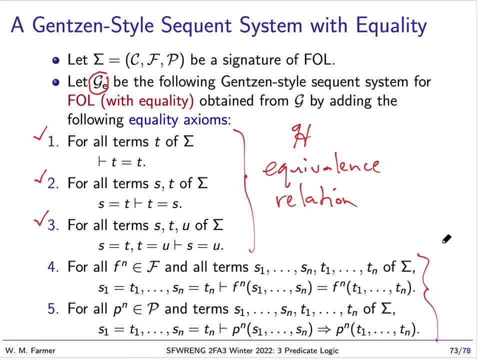 And then these last two are for a congruence. Now, if we have a congruence, That means we can substitute equals for equals, And so these two axioms are like, very like I said, very similar to the ones we had for script h. 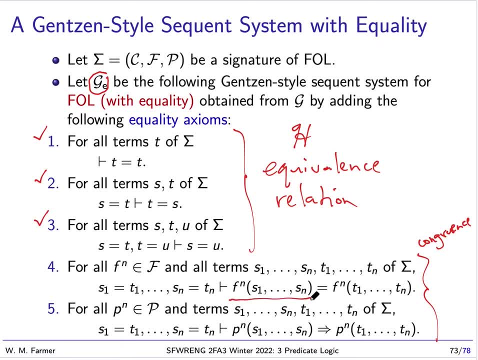 The first one says: if we have a function application and we change the arguments to new arguments, as long as these new arguments are all equal, then we'll get a new function application which will be equal to the other one. In other words, we can do equals for equals. 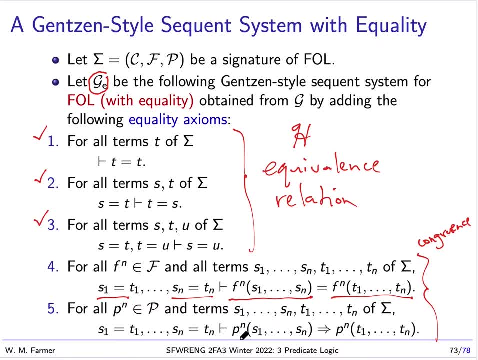 And The axiom for predicate applications is similar. If we have a predicate application and we change its arguments to other arguments that are equal to the original arguments- that's what this says- then that will imply the result of applying this predicate to those new arguments. 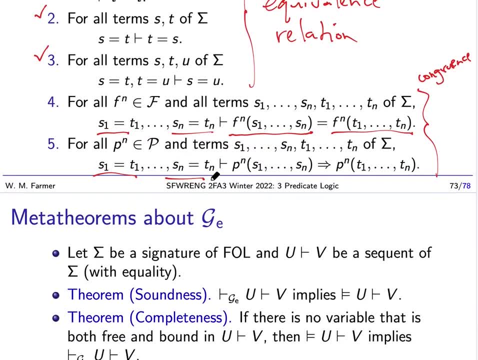 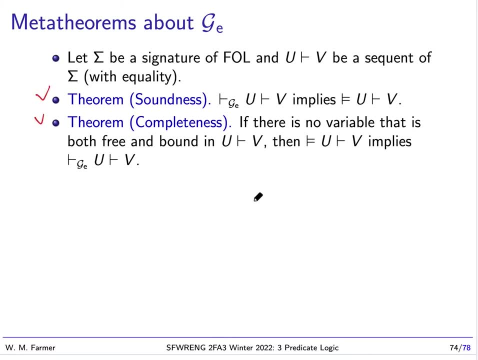 So this, this system: g sub e, it's sound, and it's It's sound and it's It's complete. Remember, g was sound and complete only for formulas that did not involve equality. g sub e is sound and complete for all formulas. 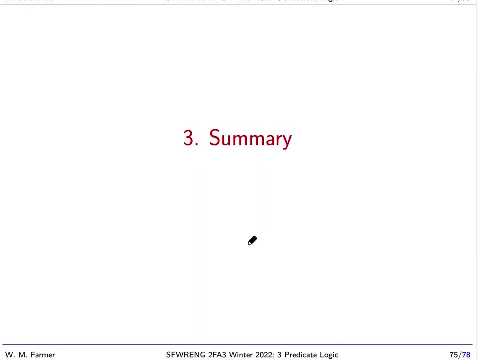 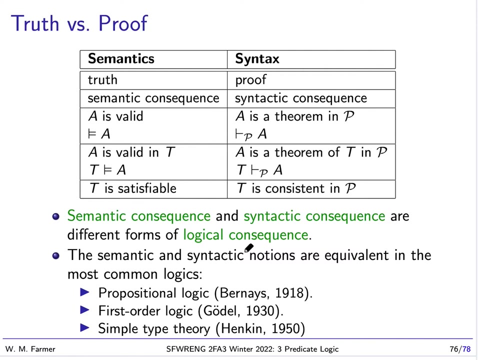 Okay, so The last part of this topic. we give a summary And I want to contrast two different kinds of notions. We have truth notions and proof notions. So truth notions are Deal with the semantics of FOL and proof notions deal with what we can prove in a proof system for FOL. 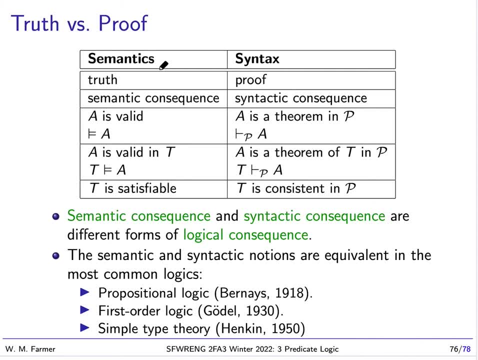 So we have this nice correspondence between these semantic elements and these syntactic elements. The reason we say syntactic here is because proving is a syntactic operation. We're basically taking expressions. these proof trees are proofs and we're manipulating them. So truth. 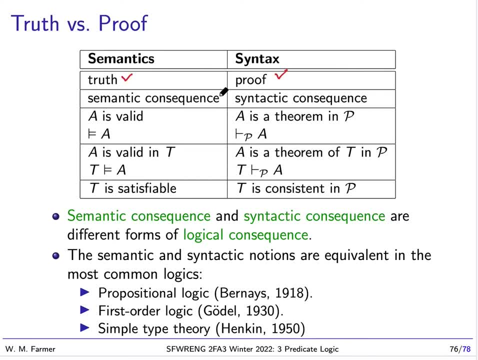 Corresponds to proof And semantic consequence corresponds to syntactic consequence. Remember, both semantic consequence and syntactic consequence are different forms of logical consequence. Then if we say that A is valid, that means it's going to get a truth value of true in every model. 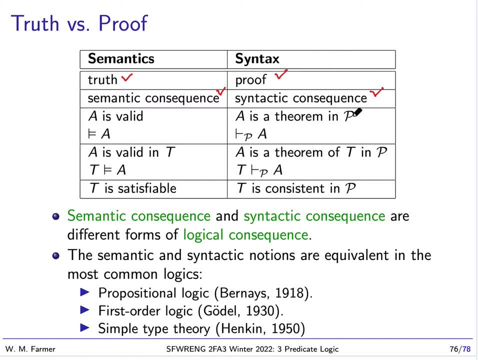 That corresponds to A as a theorem in a proof system. In other words, it's something we can prove And we can prove in the proof system from no assumptions, And in the first case we write this: This means A is valid. 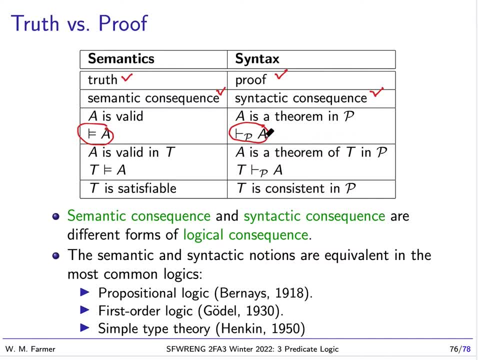 We write this. This means that A is a theorem in a proof system And then we can say A is valid in T. That corresponds to saying A is a theorem of T and P: A is a theorem of T and P means we can prove A in P using the axioms of T. 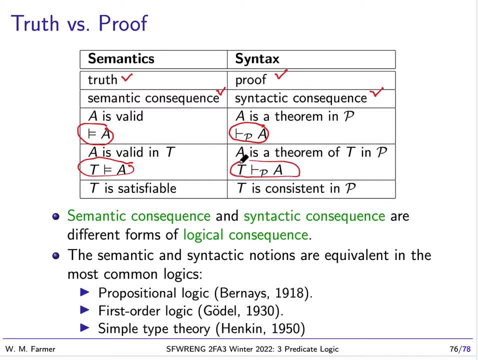 And so we have this corresponding to this, And finally we have: T is satisfiable corresponds to: T is consistent in P. T is satisfiable means T has a model. T is consistent in P means T. we can't not. everything is a theorem of T. 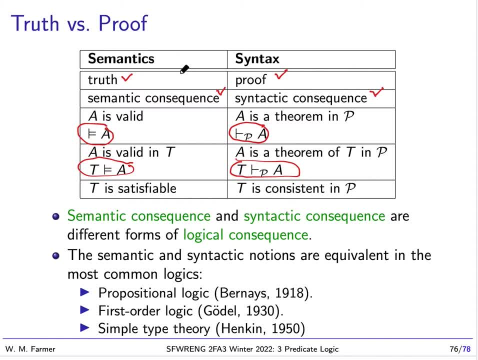 Now for some logics. these two categories of concepts are identical, So, in other words, semantic consequence is equivalent to syntactic consequence, Or another way of saying it, whenever. something will be a semantic consequence if, and only if, it's also a syntactic consequence. 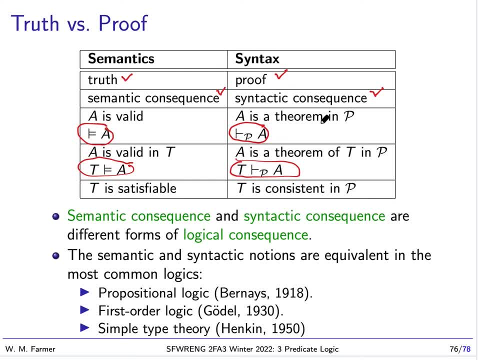 Likewise we can say that a formula is valid if it only is a theorem in our proof system. Now we can also say T is satisfiable if it only T is consistent. Now we can also say T is satisfiable if and only T is consistent in P. 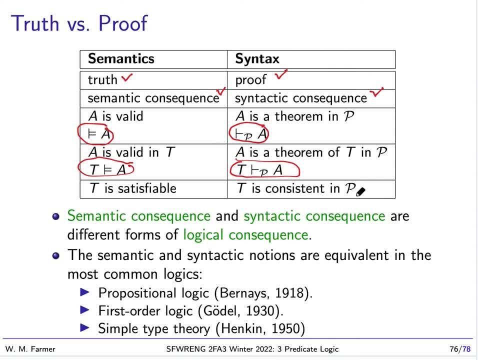 Now we can also say: T is satisfiable if it only T is consistent in the proof system. Now the logics for which these two notions are equivalent are the most common logics, our propositional logic, which Brunei showed this equivalence in 1918.. 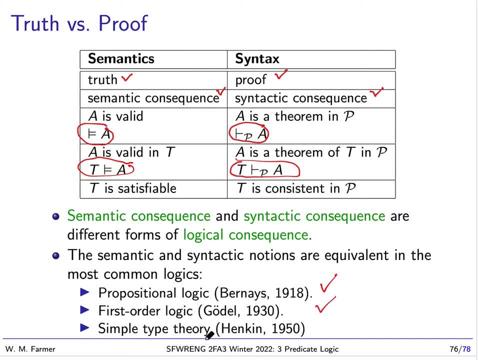 First our logic, which Guerreau showed in 1930.. And simple type theory: if you use a particular semantics Hencken showed in 1950.. And simple type theory: if you use a particular semantics Hencken showed in 1950.. 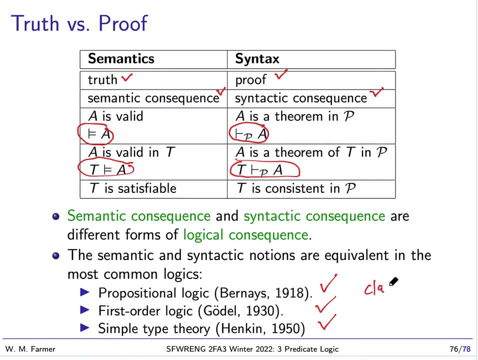 Simple type theory is what people also call classical higher-order logic. So in normal mathematics people often talk about these two different groups of concepts of being equivalent. That is not always true, but it is true for these logics, And in some logics it's not always true. 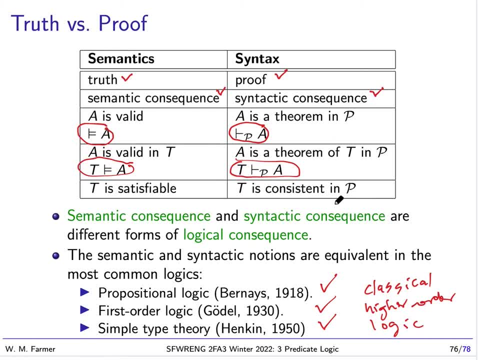 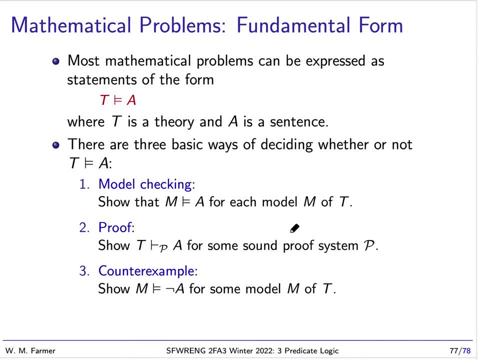 And in some logics, these notions are distinct from each other. Okay, so one more thing to talk about. This is the fundamental form of a mathematical problem. Most mathematical problems can be expressed in the following form: T, double-turn style A, and what that means is A is valid in T, which means that A is valid. 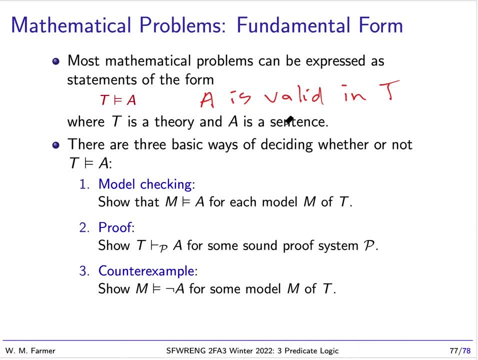 in every model of T. So most mathematical problems can be expressed in this way, and if we want to solve the problem, we really have three ways of doing it. The first is what I'm going to call model checking. That is the most obvious way, because what this means is that for every model of T, 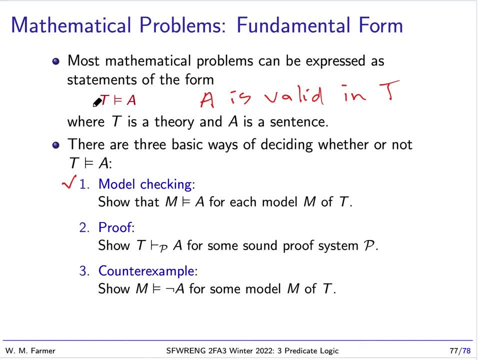 A, that model will be a model of A. The models of T are all models of A, in other words. So what we have to do With model checking is we check that A, that that if we have a model of T,